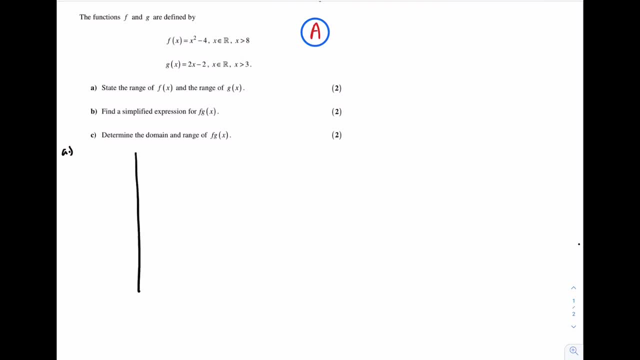 Let's start off with a graph of f of x. Here is the sketch of y, equal f of x. for x is greater than 8.. Notice that there are dash lines for x is less than or equal to 8.. Those dash lines are not included as part of my sketch. 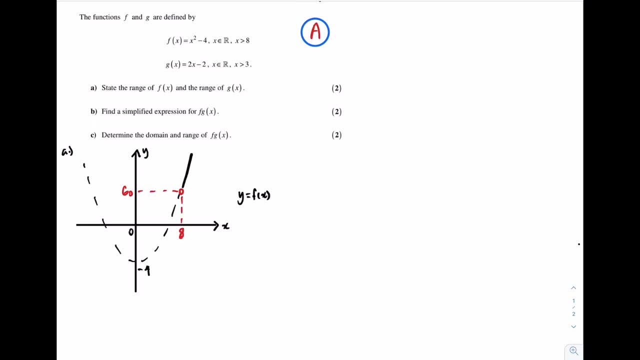 Now to find the range of y equal f of x, I need to focus on the y axis In particular. I'll be looking at this portion over here. So what is the range of y equal f of x? Well, the range of y equal f of x is just: f of x is greater than 60.. 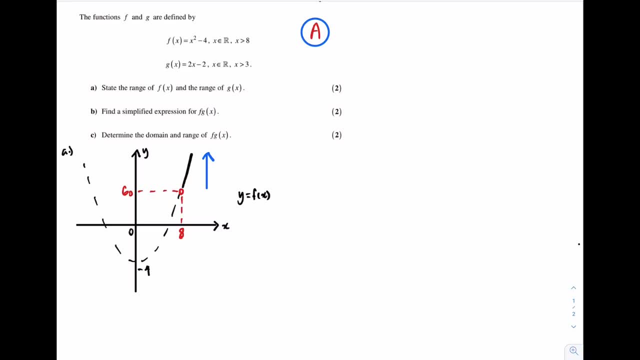 Notice that we have a circle. We have a circle over here because x equal 8 is not included in the domain. Hence y equal 60 is not included in the range. So the range of f of x will just be f of x is greater than 60.. 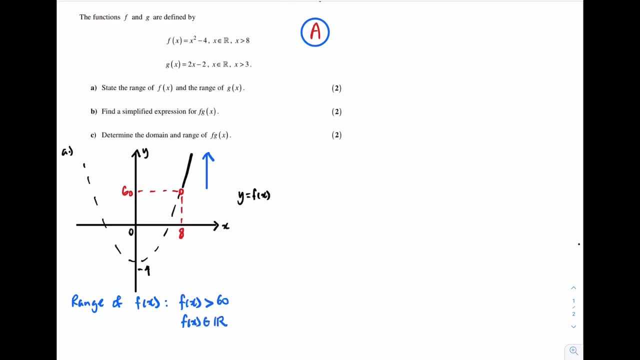 f of x is an element of the real number set. Now I'm going to sketch the graph of y equal g of x In order to determine The range of y equal g of x. So here is my sketch of y equal g of x, for x is greater than 3.. 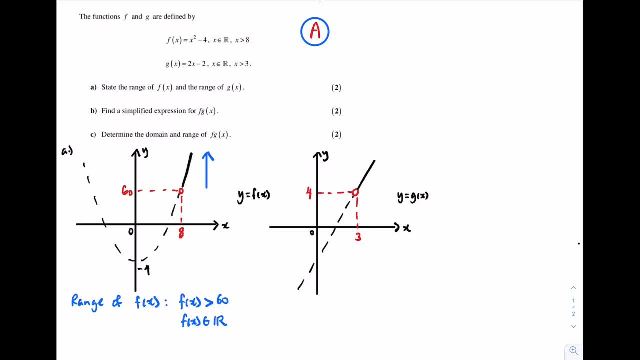 The dash lines are not included as part of my sketch. Notice that We have a circle over here because x equal 3 is not included in the domain. Hence y equal 4 is not included in the range. Now, to find the range of y equal g of x, I need to focus on the y axis. 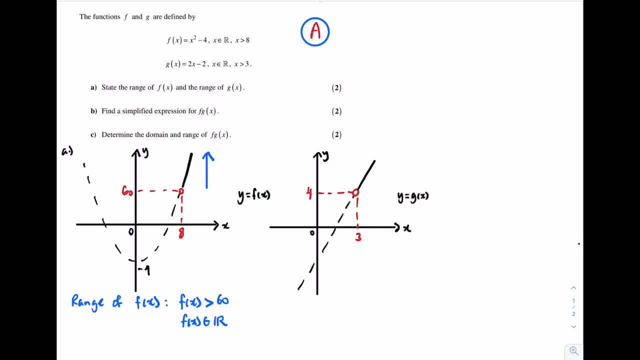 And in particular I'll be looking at this portion over here. So the range of y equal g of x for x is greater than 3 will just be g of x is greater than 4.. Range Of g of x Is g of x is greater than 4.. 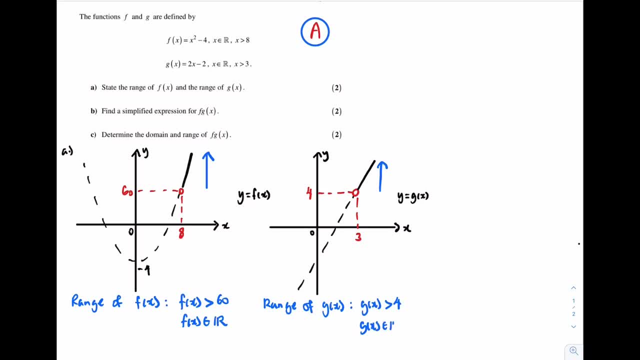 g of x is an element of the real number set. Let's have a look at Part B. For Part B, I need to find a simplified expression for f of g of x. So f of g of x, Firstly, can be rewritten. 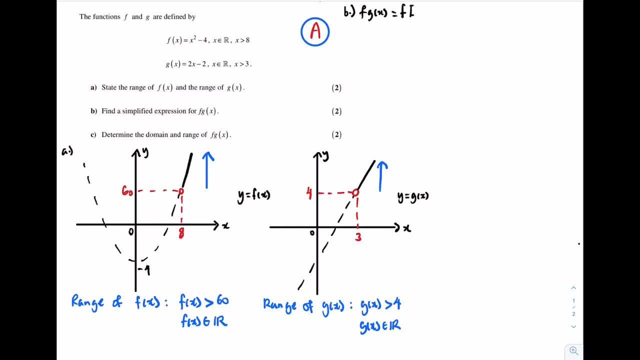 So f of g, of x as f. What does this tell us? Well, the input for f is g, So I can replace the g with 2x-2.. Now f is just f, but with the x's replaced with 2x-2. So I have 2x-2. Now, this is a quadratic in. 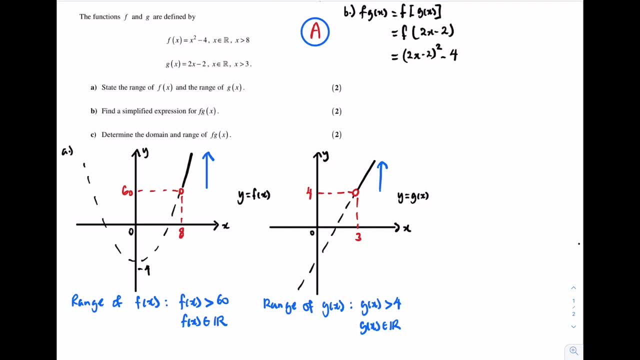 vertex form. When we have a quadratic in vertex form, we can read off the turning point. The turning point for this particular quadratic will just be To find the x coordinate of the turning point. we need to set whatever we have inside the bracket equal to zero. so if I set 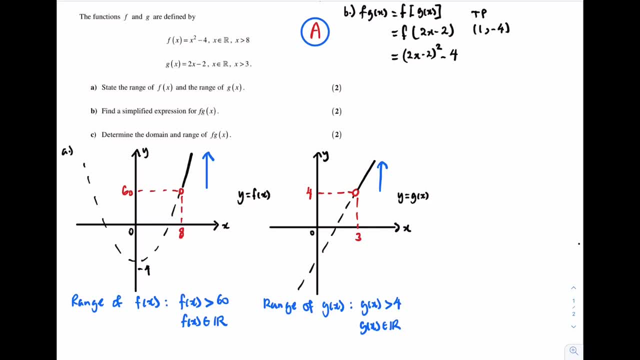 2x-2 equal to 0 and I solve. I get x equal to 1.. The y coordinate of the turning point is the number that you have outside the bracket. In this particular case, it is minus 4.. To get the final mark, I need to simplify this. 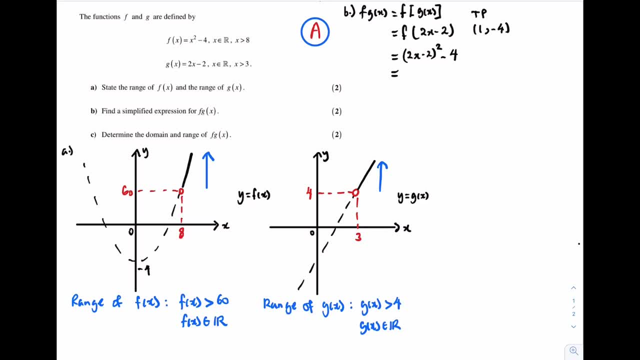 expression. So if I expand and then simplify I obtain the result 4x squared minus 8x. Let's have a look at part c: Determine the domain and range of f of g of x. I'm going to start off with the domain of f of g of x To find the domain of any composite. 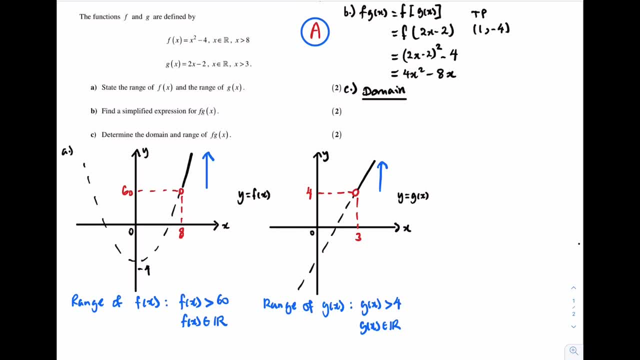 function. it is always useful to draw a mapping diagram. My first set will represent x. x gets mapped onto g of x, which is my second set. The domain for g of x is x is greater than 3.. g of x then gets mapped onto f of g of x, which is my third set, The domain 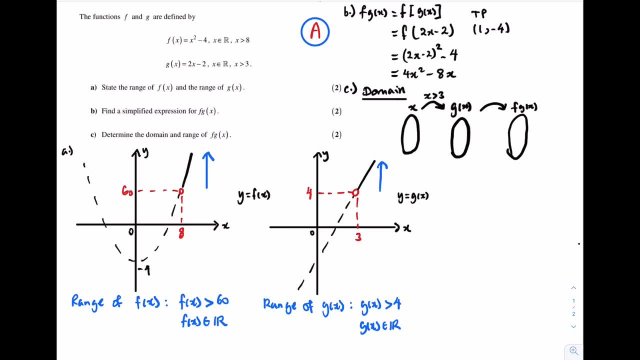 for f is x is greater than 8.. Because the input of f is g of x, I need to write g of x, as I know that g of x is 2x minus 2. So I can set 2x minus 2 to be greater than 8.. I need: 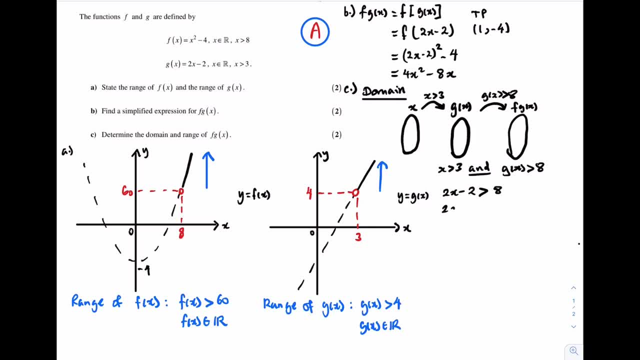 to now solve this inequality. So I get: 2x is greater than 10.. Hence x is greater than 8.. I must have that x is greater than 3 and x is greater than 5. So I can write: x is greater. 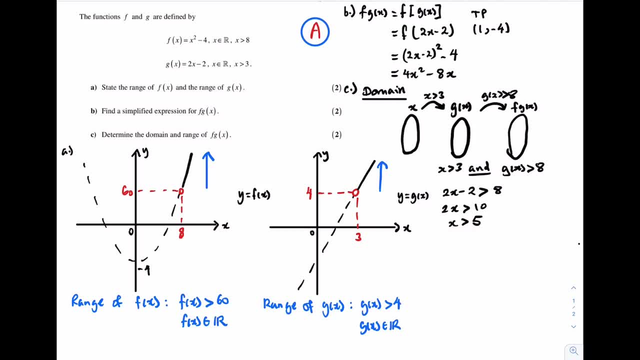 than 5.. What is the overlap? Well, the overlap is just: x is greater than 5.. Hence, the domain is: x is greater than 5.. x is an element of the real number set. Let's have a look at the range of f, of g, of x. 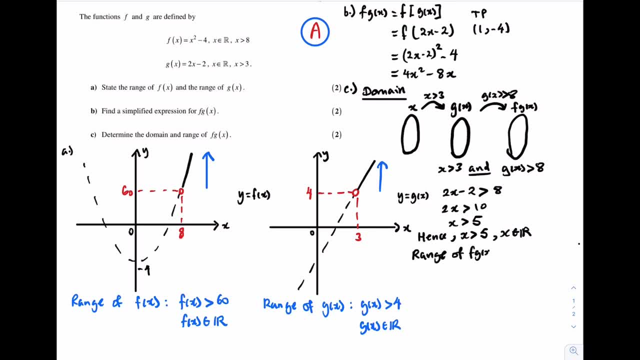 To find the range of f of g of x. I'm going to sketch the graph of f of g of x for its domain, which is x is greater than 5.. Here is the sketch of y equal f of g of x for the domain x is greater than 5.. Notice. 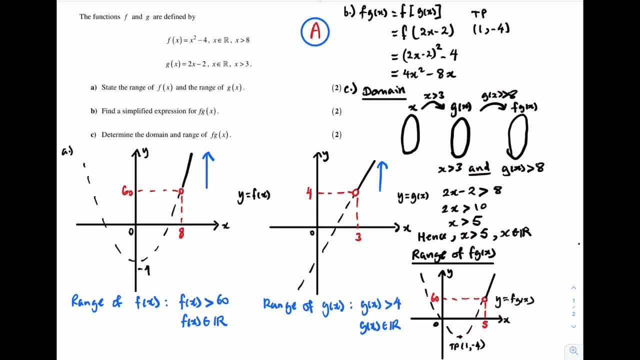 that the dashed lines is not included as part of my sketch. There is a circle at this point because x equal 5 is not included in the domain. hence y equal 60 is not included in the range. Going back to the circles. If these circles were shaded, 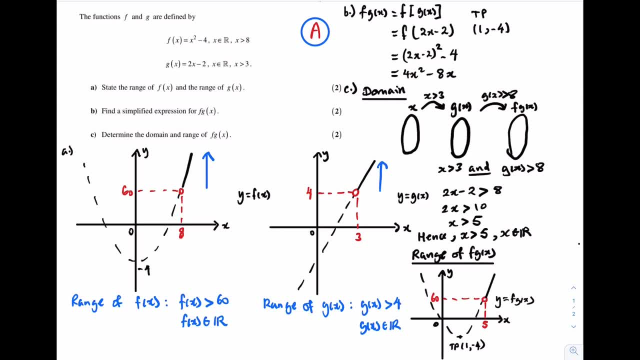 Then the corresponding x values will be included in the domain and the corresponding y values will be included in the range. I thought I'll mention this important fact. Okay, so, to find the range, I need to focus on the y axis In particular. I'll be looking.